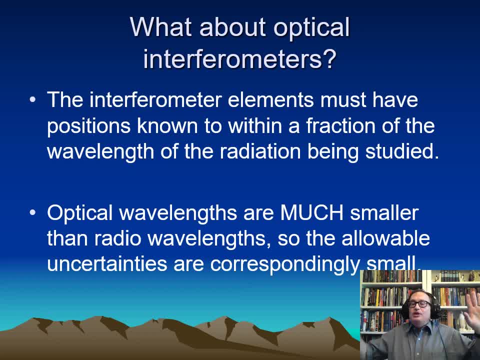 do For radio telescopes. you can do this with radio telescopes that are pretty far apart. For optical telescopes they actually have to be so close together. you can actually fire a laser between them and use the laser to do that. So if you're using optical telescopes you can do this. 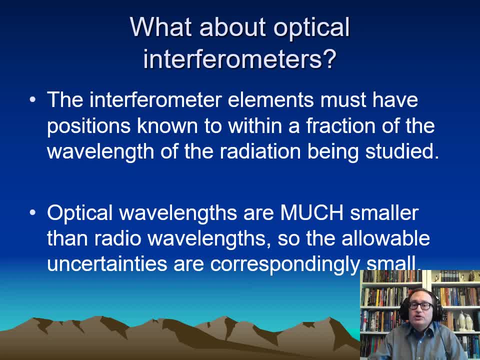 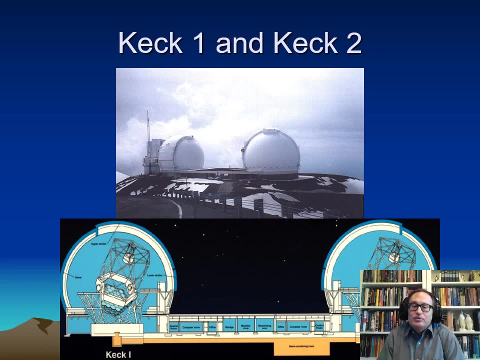 with a laser and interference of the laser itself to measure that distance to that level of precision. So that means that you are limited to much closer instruments and it's much harder to make that work. Well, guess what? We have made it work though The Keck telescope. We have Keck 1. 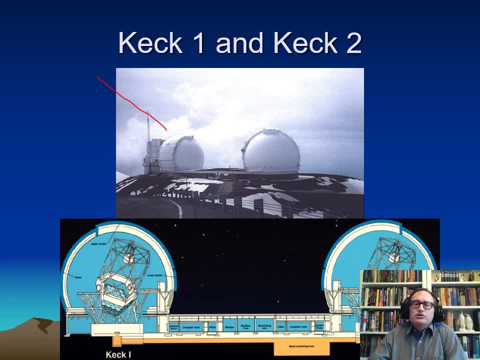 and Keck 2.. Now Keck 1 can look at something and Keck 2 can look at something else, and that's no problem. So we can have two of these giant telescopes looking at each other, and that's. 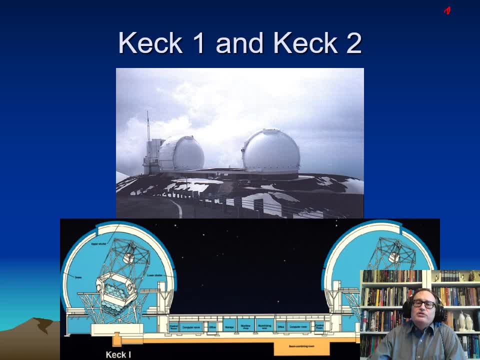 no problem. So you can have two of these giant telescopes looking at things, or you could have something up here and Keck 1 and Keck 2 look at the same object and now the light of one of them can be fed underground and light of the other one fed underground and then put together in the 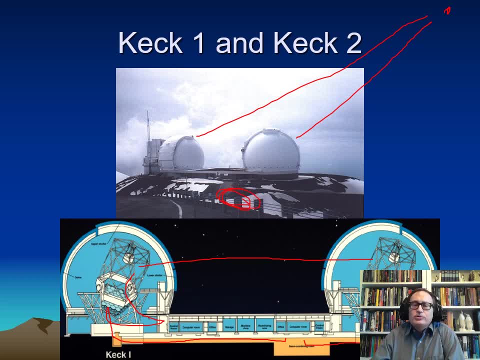 laboratory underneath, and now you have an optical interferometer that simulates each one of these as a monster telescope, and now you can simulate the resolution of a telescope that big, and so that's going to be much, much, much better. It doesn't work all the time. Most of the time. 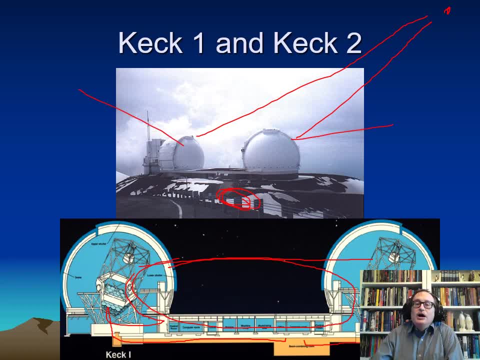 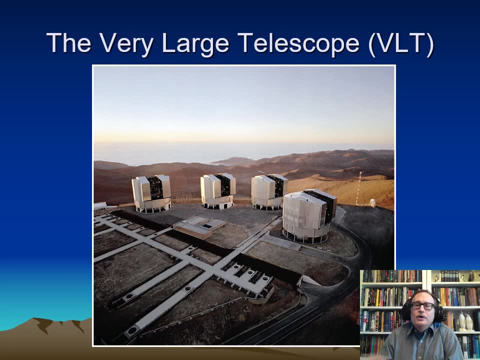 you're actually going to use each telescope as an individual telescope, but once in a while you can throw them together and get much, much higher resolution if you need it. Well, in South America, the European Southern Observatory has built a facility that is four. 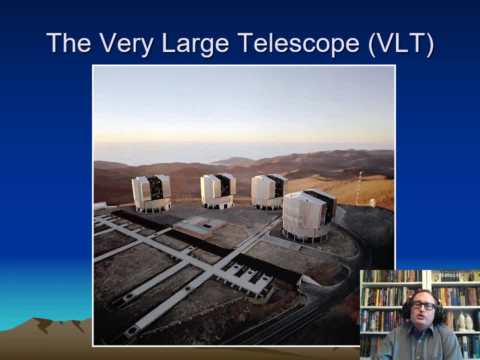 individual telescopes that strung together, can simulate one very large telescope. So what do they call such a facility? Well, duh, the Very Large Telescope. Okay, and so remember, it's astronomers naming stuff. and so the Very Large Telescope is actually four different. 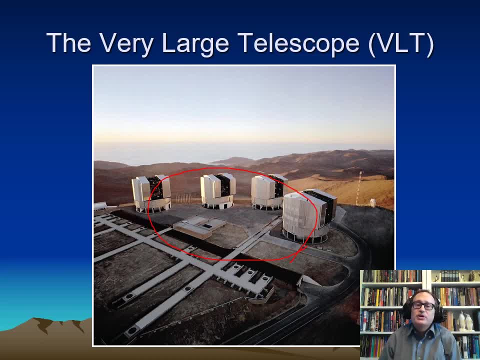 telescopes that can look at four different things, or they can all look at the same thing and simulate one very large telescope, and so that's in fact they've, since they've actually added a couple outrigger telescopes out here that actually simulate even slightly larger. 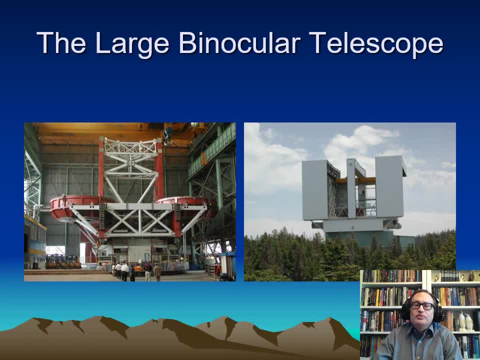 So that's an example of an optical interferometer. The Large Binocular Telescope in Arizona is another example of an optical interferometer. So here it is being constructed, right here, and there's the facility right here where it's being built, and so it's going to act like- even though you have two mirrors here, it's going to act like. 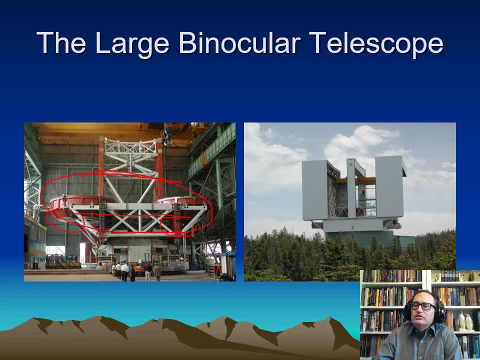 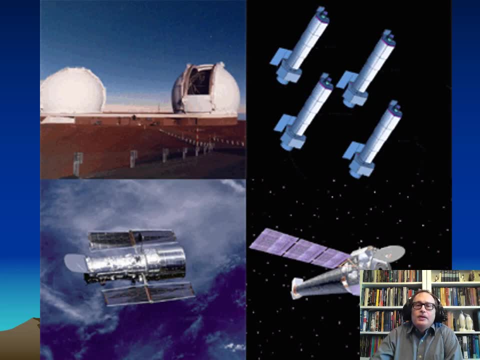 one big telescope of that size right there. Okay, so again, this is an example of optical interferometers. Now, the CAC is a good example, but what we would really like to do is have like a fleet of space-based telescopes that can be stretched out over miles. You know, imagine you've got laser. 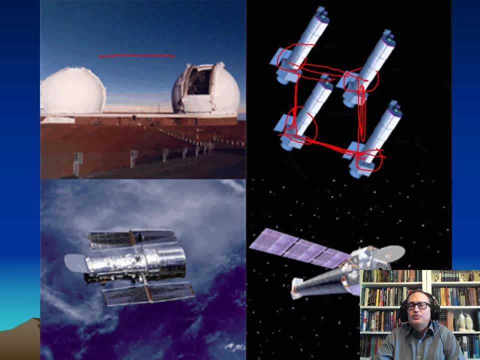 links between them all. so you know the exact position of all: the fraction, a tiny fraction of of a millimeter, a fraction of a nanometer. even So, we're trying to find out. use that and then that would actually allow us to simulate, maybe an. 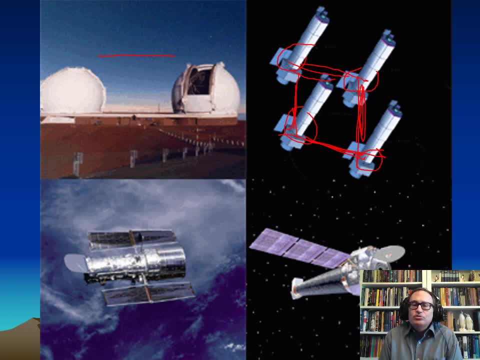 optical telescope that is miles across or maybe even hundreds of miles across. Such an instrument using optical light could actually resolve a planet around another star and resolve it clearly enough. you could actually see if there's continents on it and maybe if those continents have. 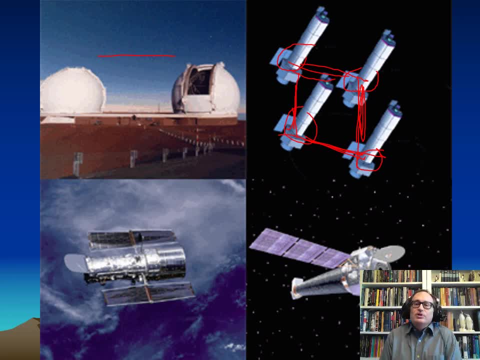 uh, evidence of greenery indicating life, And so that would be. in fact, NASA's been talking about building something called the Terrestrial Planet Finder, which is a very large space-based interferometer- uh, but they've never been approved money to do that. But that would be the. 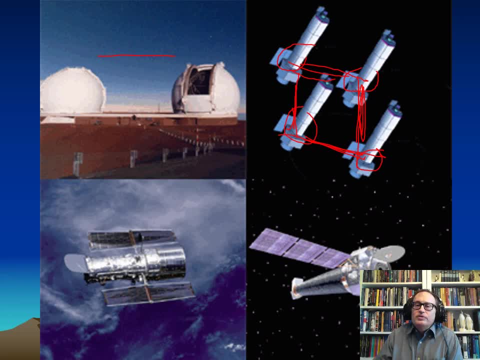 capabilities of such a space-based interferometer. Uh, so that's, that's kind of what we're looking at into the future, you know, to supplement our other space-based telescopes. Uh, so with this, this kind of gets to the end of what we're we're talking about with telescopes. uh, just tie, tie it.